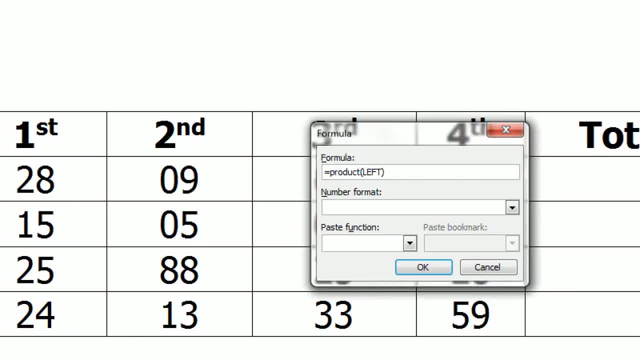 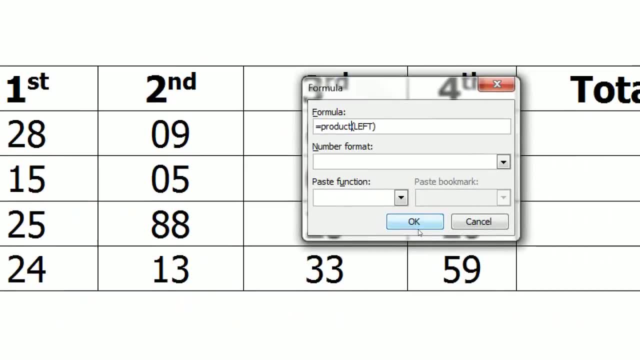 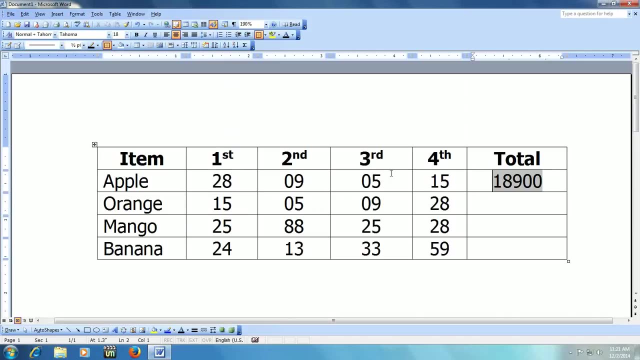 change this one like product. That's it, Product from the left side, because I have the value in the left side and press OK, Look at that, I will show you. Wait a second. You can see here the total value And the next column I will show again. To go to formula, press Alt, A, O and here I will change the. 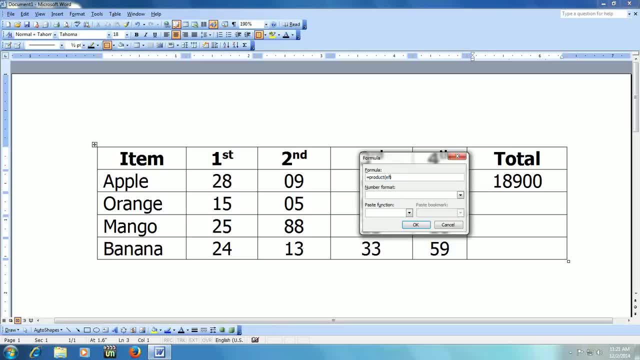 formula and I want to do from the left side, So type the left, That's it. So like this you can do some also. So if you want to do to sum, go to formula Alt A O and here already given the sum formula. So just press Enter, Look at that And the next column: if you want to do the same thing, go to Alt A O, and here you have to change because it is given the sum. But here you can see the above. It means if you want to do the same thing, go to Alt A O, and here you have to change because it is given the sum. 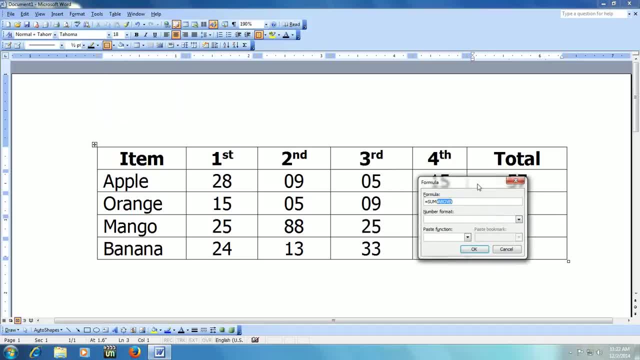 The formula will take from the above. but we don't want to take above, We want to take from the left side. So here just change the left and press OK, That's it. So like this you can do all products, minus or divided or percentage or anything of the calculation you can do easily. 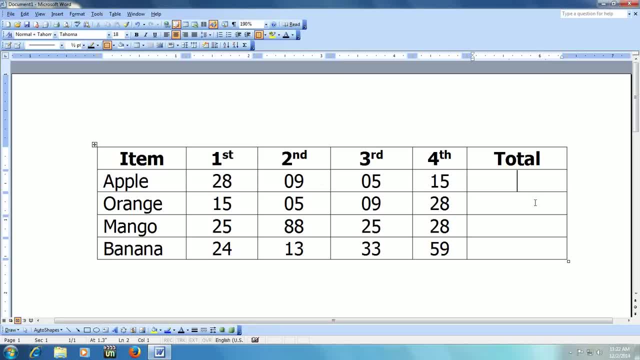 But in the first time, in the beginning, you feel some difficulty. but if you go to some practice up to two or three days, you will do very fast And I will show you if you are getting the difficulty. I will show you other method to do this. So first we will do product Go, alt, AO and just delete this. 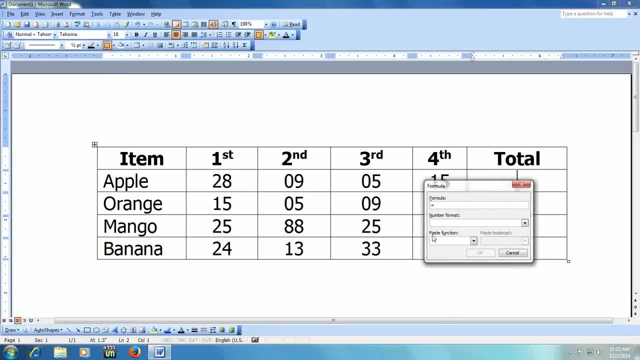 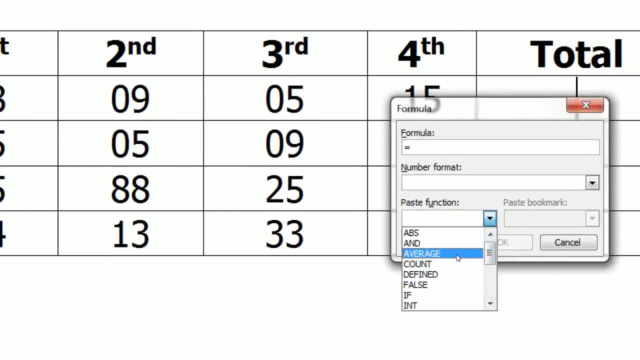 OK, Just delete this. And here you can see paste function. In the paste function, just extend this And here get the ready made formula And just delete this. And here you can see past function And here you get the ready made formula. 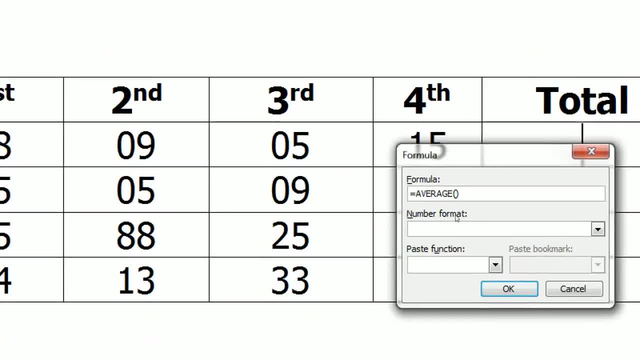 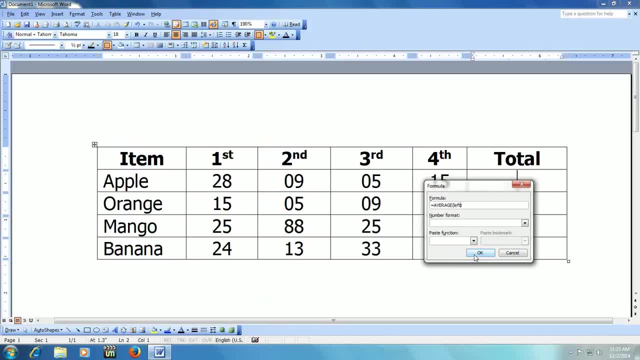 want to do average. just click on here. you can see the address and it's come. tap the here from the left. you can see left and now press enter. look at that. so like this, you can change any formula by giving the particular your product or some round like this and some like this. so I will show one more easy method for.